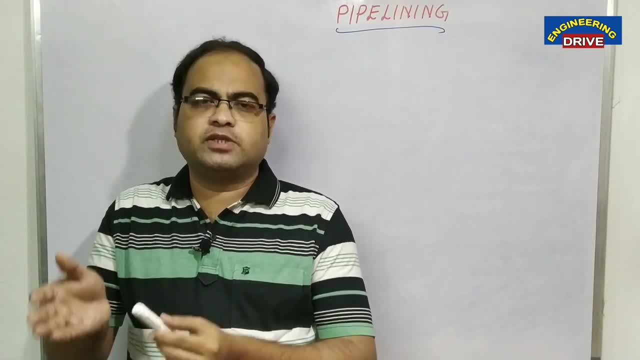 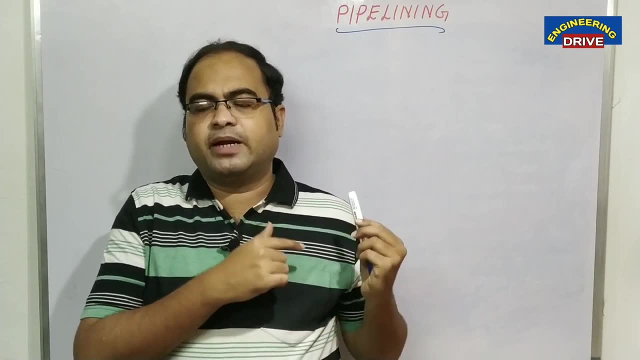 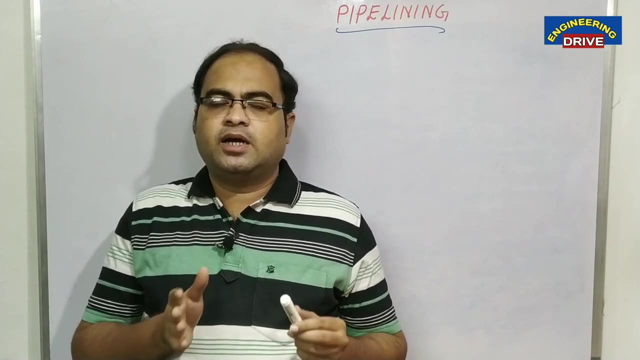 multiple programs. multiple programs means multiple set of instructions. then automatically the speed of our computer will increase. so because of that concept, only pipelining will be implemented by our systems. okay, now i will give one example to you, so that you can understand the importance of pipelining. if we use pipelining, what happened without pipelining? what is the drawback? 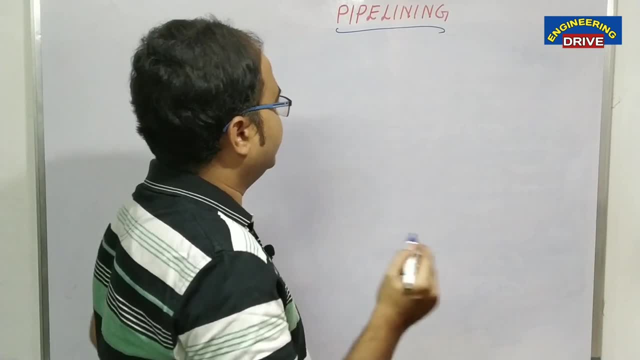 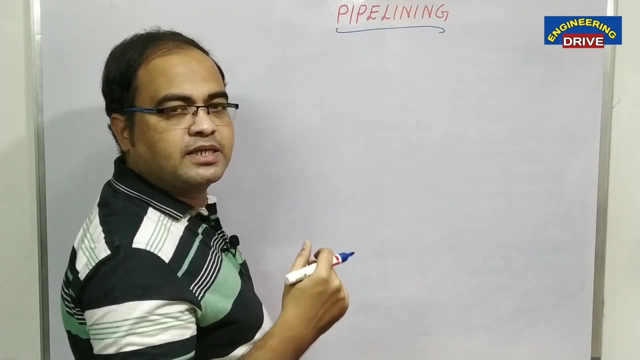 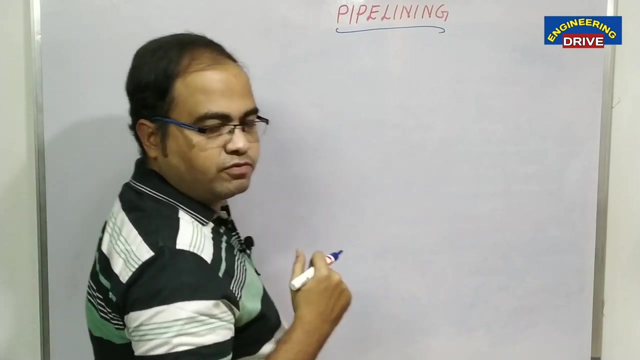 that will come in our computer. let me tell one example now, my dear students generally, how our computer executes the programs. now, what is a program? program is a set of instruction. program is a set of instructions. you know that in instruction there are three major steps for the execution of instructions: fetch the instruction, decode the instruction and execute the. 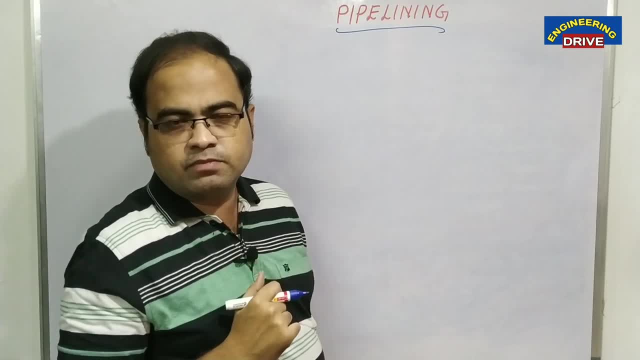 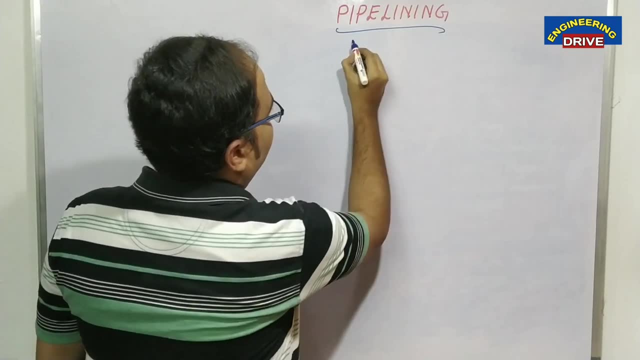 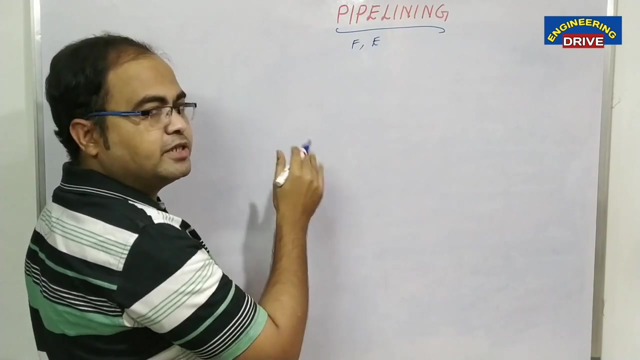 instruction combined together. we call them as instruction cycle. okay, now let us take two primary steps for the execution of one instruction. first step: i am taking it as a fetch instruction, fetch the instruction. second step i am taking taking as a execution of instruction. these are the two. 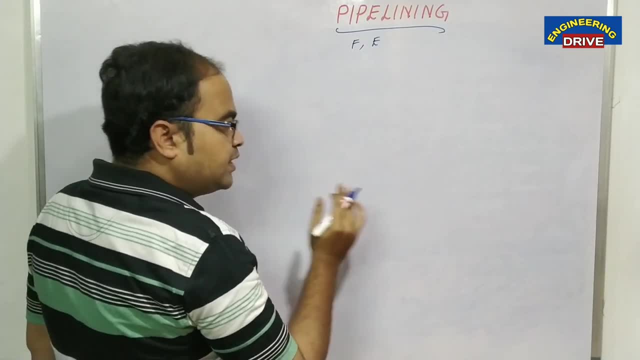 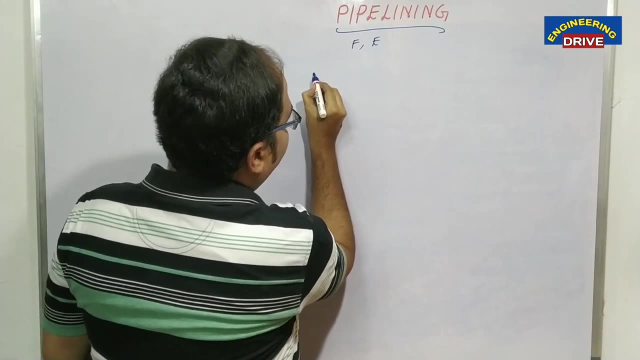 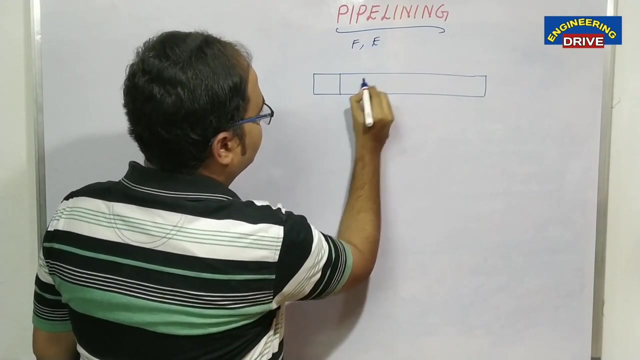 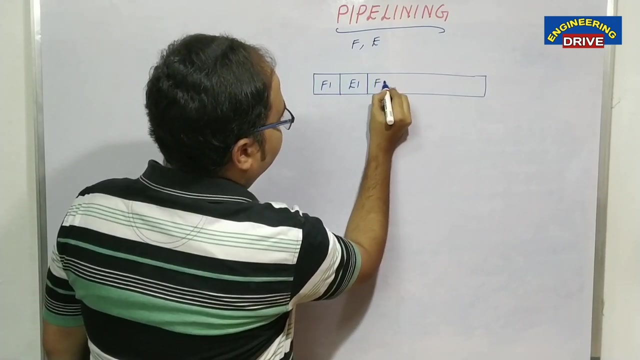 primary steps i have taken, for my simplicity now, what our computer will do generally without pipelining, that i will explain first. okay, see here, let us take, let me draw one simple diagram to you. let us say: f1, f1, f1 is f1, f1, f1, f1. this is f2, f2. this is f3, f2, f1. this is f2, f1, f1, f1. this is f2. 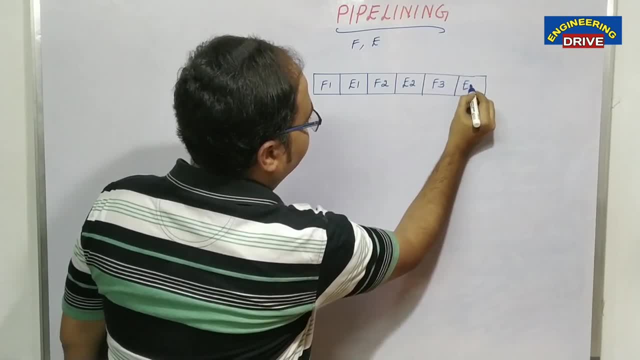 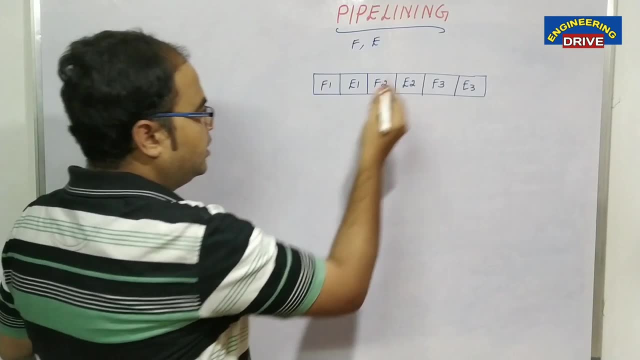 this is f1, e1, this is f2, e2. okay, this is f3 and this is e3. okay, sir, what you have done, what you have written in this diagram. you can ask question to me. let us say: f1 and f2 are nothing, but. 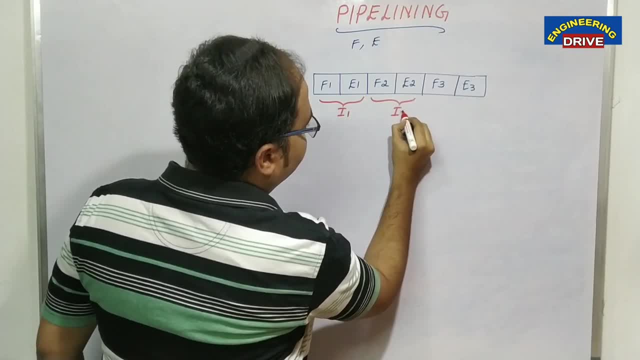 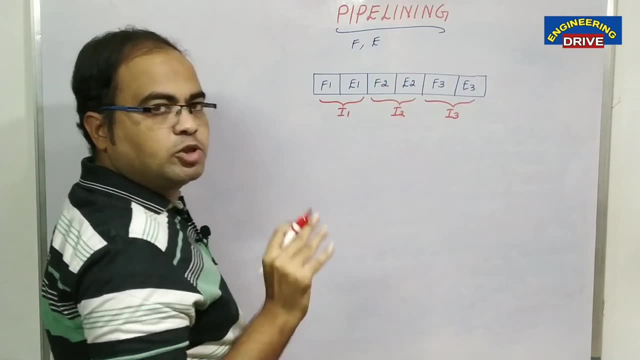 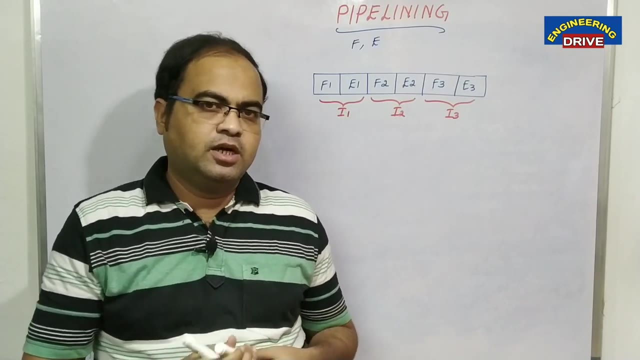 F2 and E2 belongs to instruction 2, F3 and E3 belongs to instruction 3.. So how many instructions I want to execute? Three instructions I want to execute Now our computer without pipelining how it will execute these instructions. 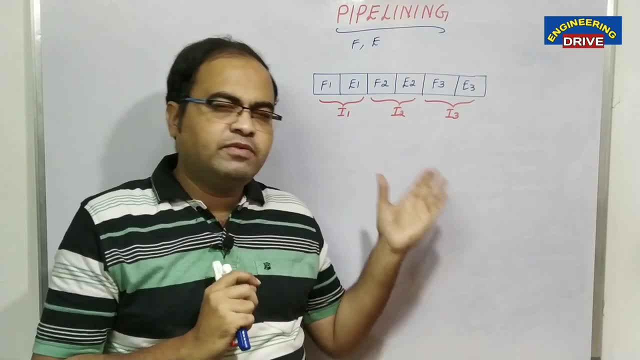 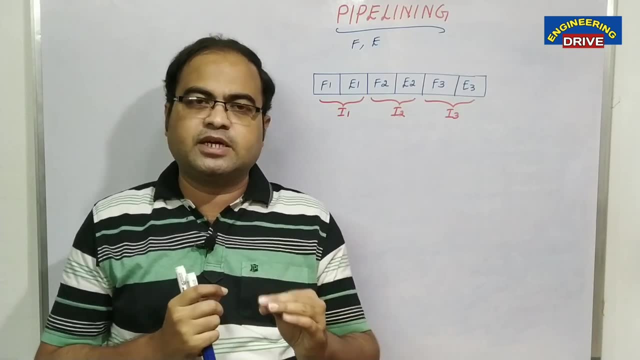 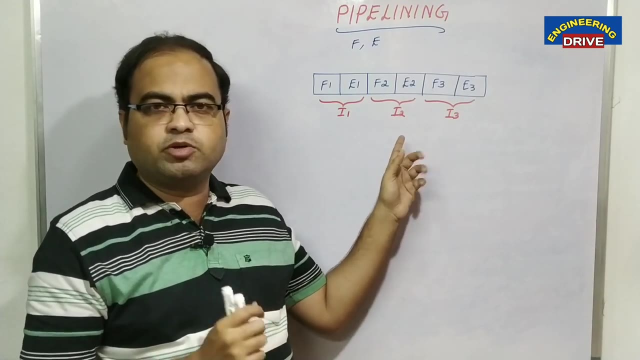 Let us say our program has three instructions. when we can say our program will be executed, if all the three instructions are executed, then we can say our program is successful executed. Now, in order to execute this single program, how many instructions should be executed? 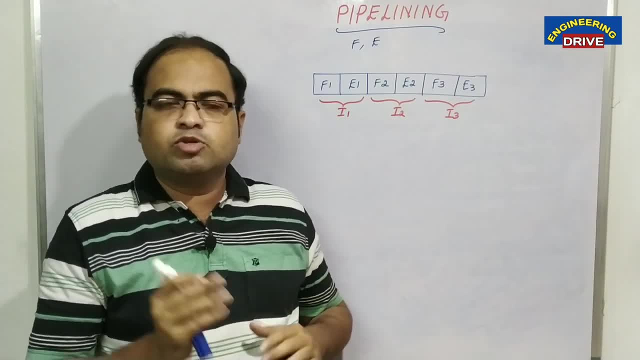 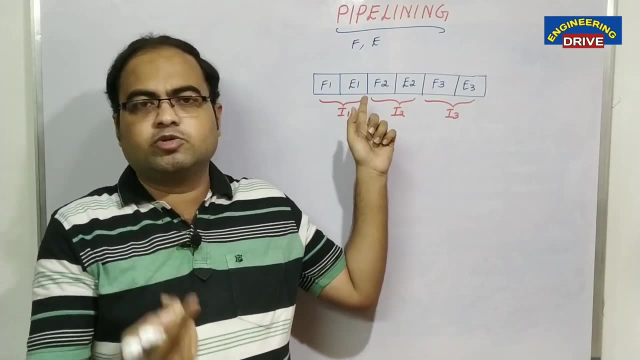 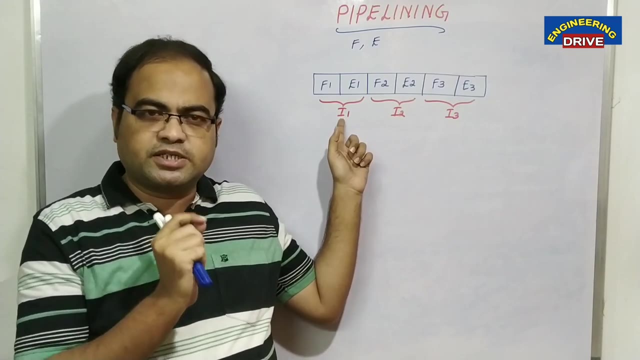 Three instructions should be executed: I1,, I2 and I3.. So what our computer will do generally, you know. first of all, F indicates fetching the instruction, E indicates execution of instruction. F1 means fetching the instruction 1,. first of all, our computer will fetch the instruction. 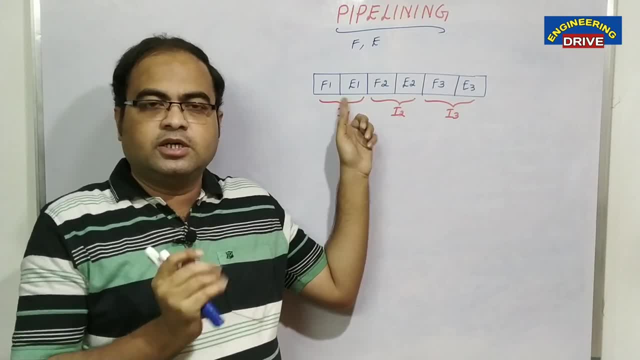 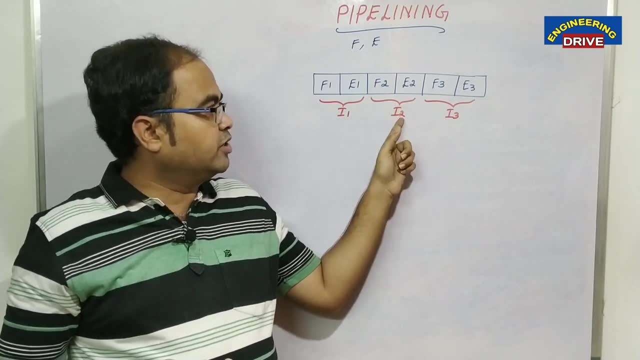 1, then it will execute the instruction 1.. First instruction 1 is executed. So what is the instruction 1? Fetching successfully. then it will go to the second instruction, I2, fetching of I2, execution of I2.. 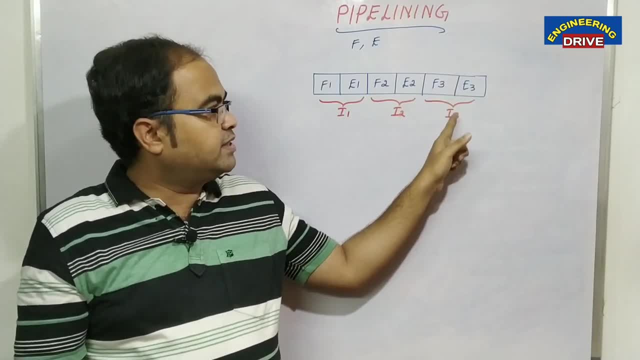 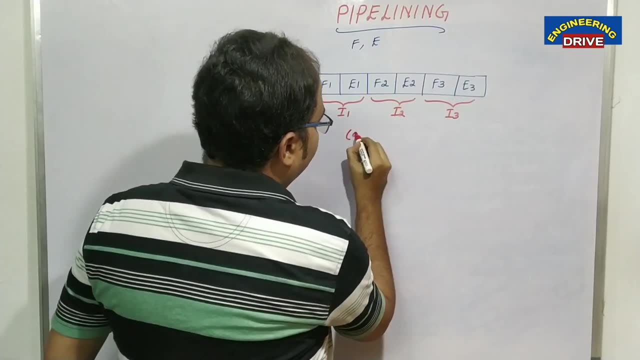 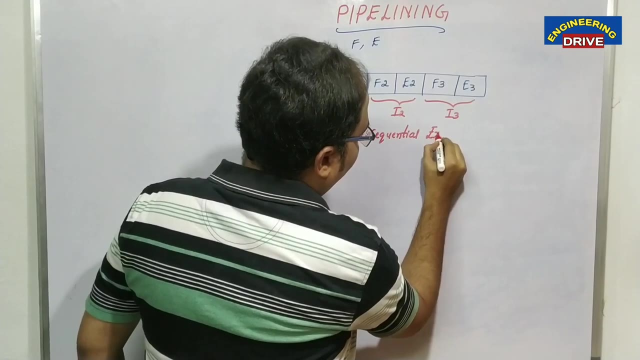 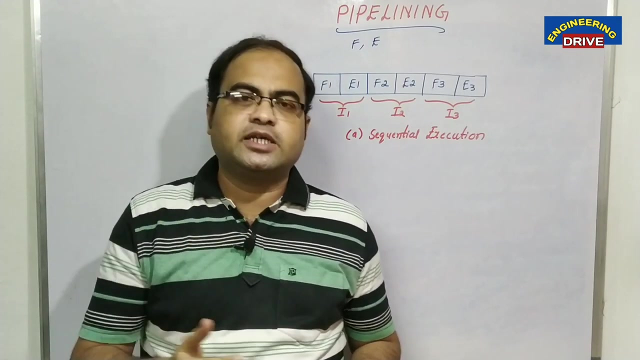 Once I2 is completed, it will go to the third step: fetching of I3, execution of I3.. So we can call this concept as- let me take this first example- this is a sequential execution. It generally employs sequential execution of instructions. 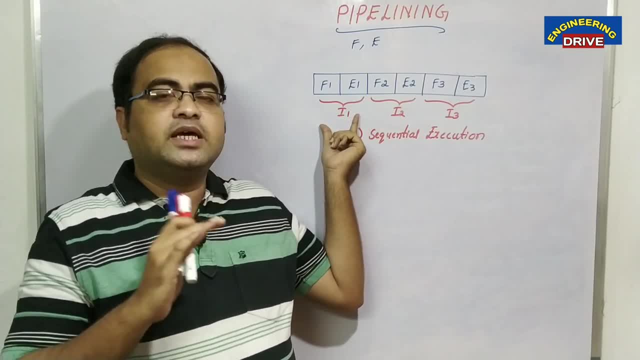 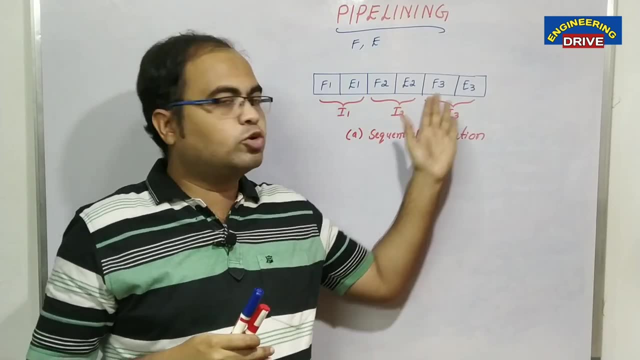 So why I am saying sequential execution: first instruction 1, then instruction 2, then instruction 3.. Let us say: if our program has some more instructions, then control will go to those next instructions. Now what is the drawback in this method? 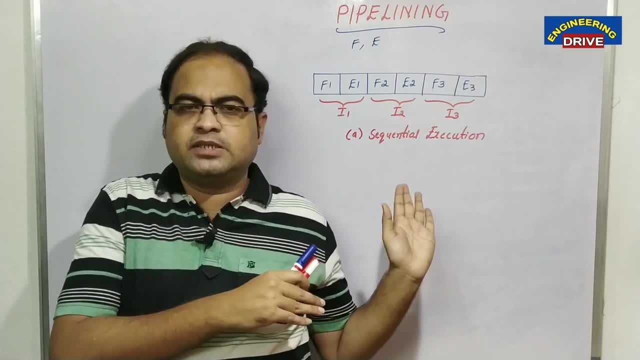 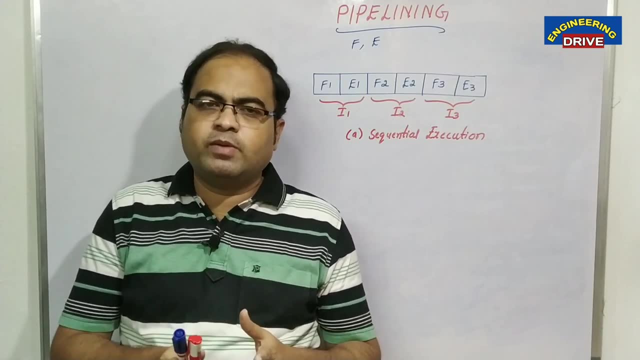 The drawback in this method is even though it is a very cheap method, which means there is no need to have expensive hardware in this. but the big drawback is speed of execution. the performance of the program, The performance of our computer becomes considerably very slow. ok, why? 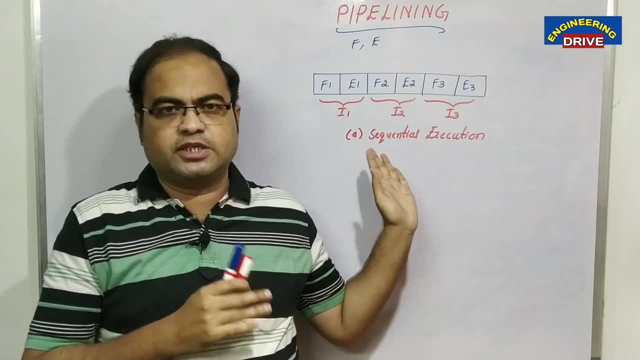 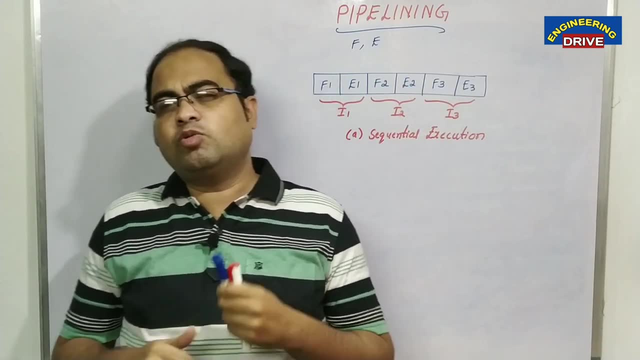 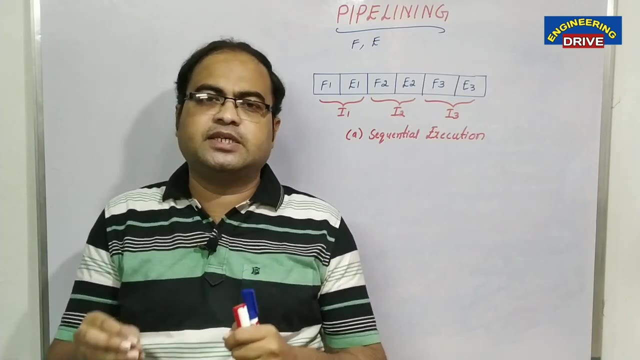 Because our computer generally employs serial execution of instructions, sequential execution of instructions: instruction 1,, instruction 2,, instruction 3,. ok, Now how I can improve the performance of my computer, now how I can execute multiple instructions or concurrent executions at the same time. the answer is pipelining concept. 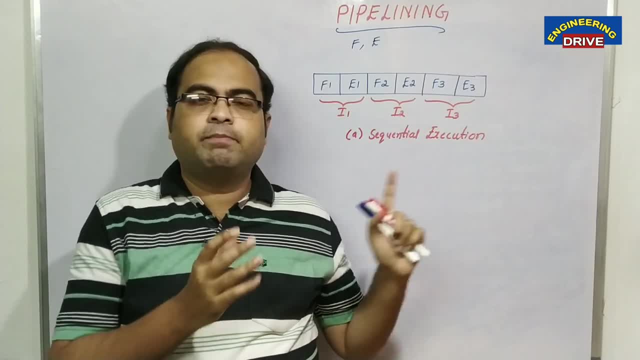 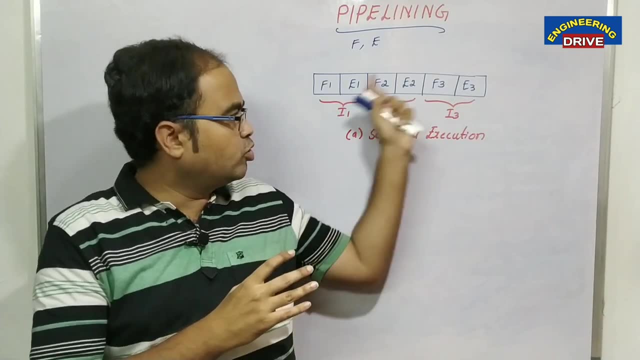 Now. we need to introduce pipelining now because of this problem: Pipelining. Pipelining concept has been introduced and our computer will make use of it. ok, How pipelining will work. So hopefully the first diagram has been clear to you, ok. 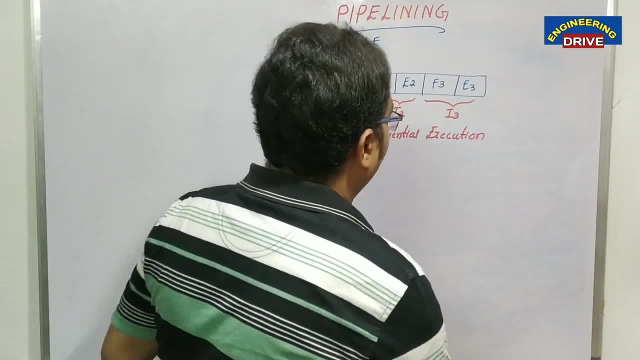 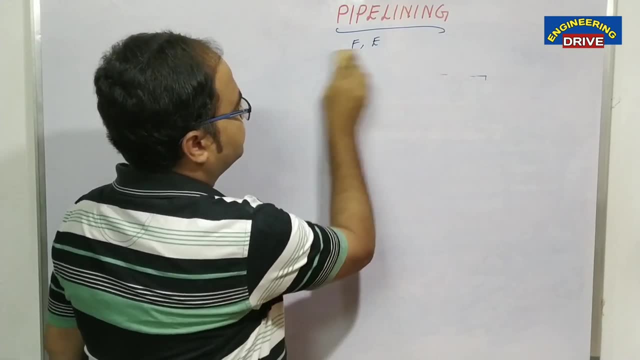 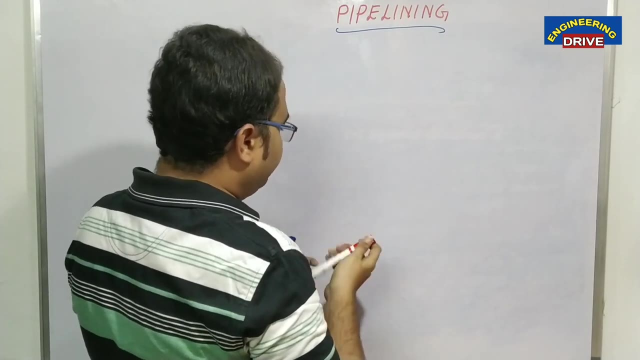 If you want, you can note down this diagram. ok, pass the video. I can note down the diagram. Let me erase this one. this is sequential execution Now, what I am going to do means: let me erase this Now. I want to implement pipelining concept now in my computer. how I can implement the? 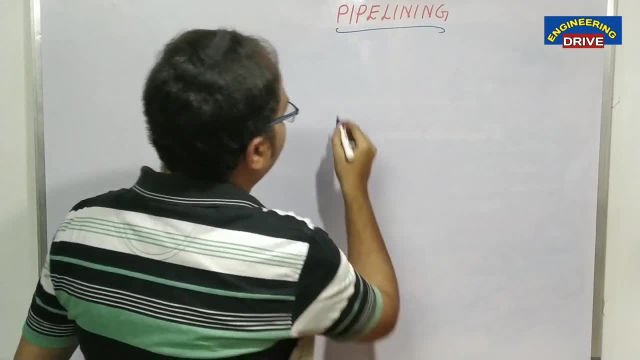 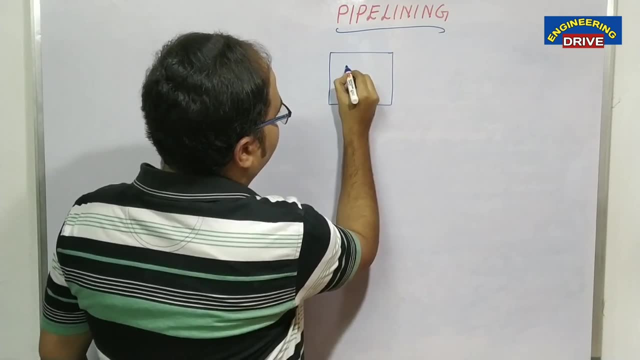 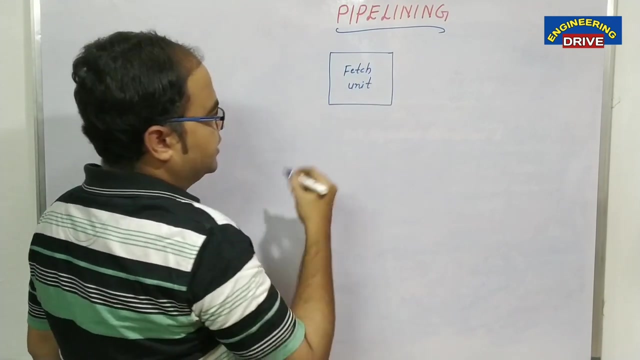 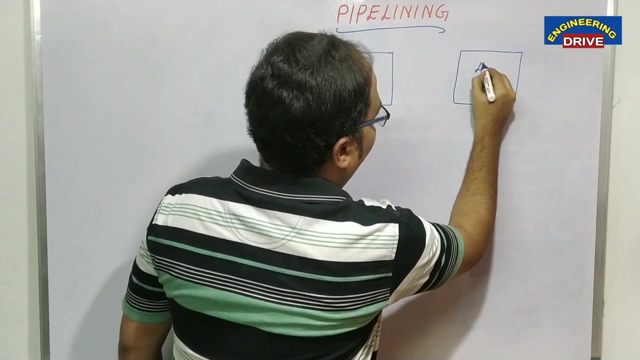 pipelining concept, I need to have two separate hardwares. first, hardware is nothing, but it is used for it is a fetch unit or fetching of instructions, whereas the second hardware that I am going to make use of is for execution unit. 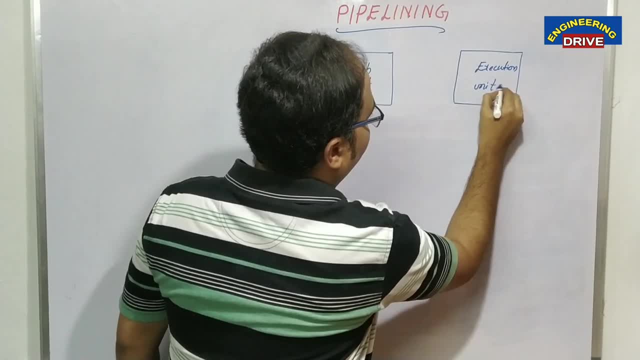 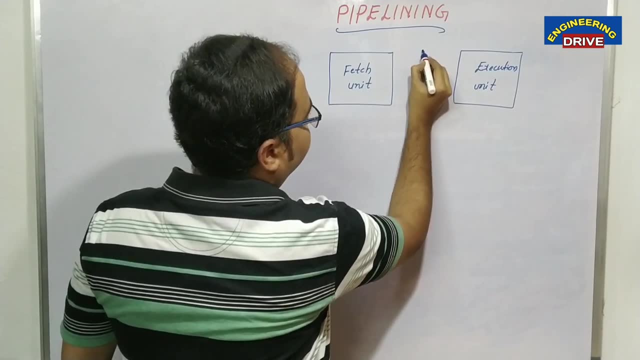 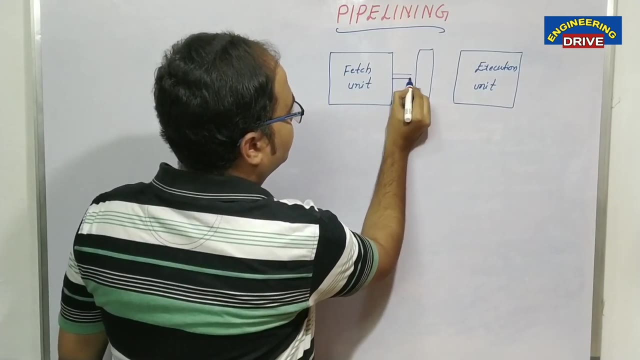 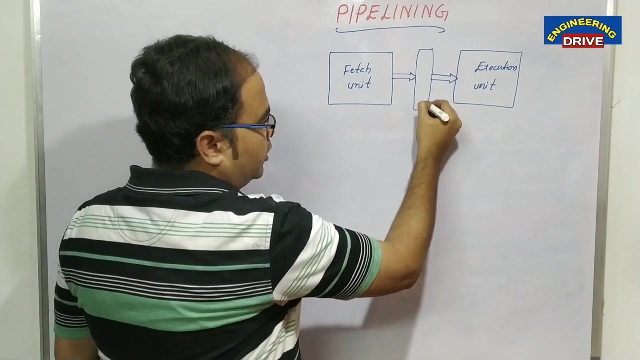 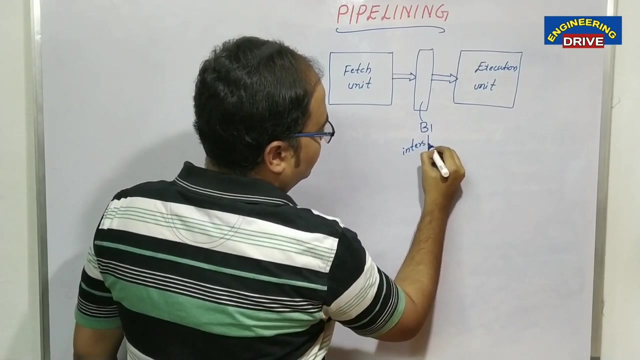 For fetching: Ok, Ok. Ok, For fetching of instruction: separate hardware. for execution of instruction: separate hardware. ok. And there comes this middle important point. This is known as- let us say, I am calling it as- B1, this is our inter stage pipelining. 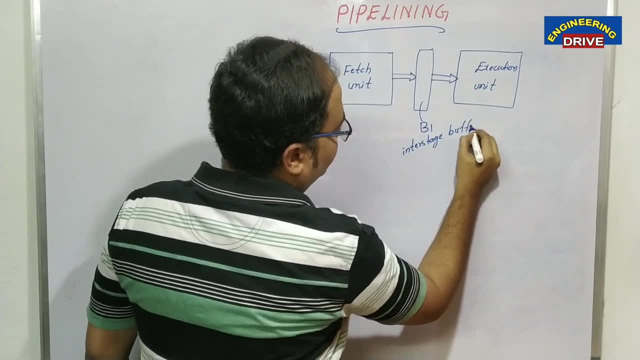 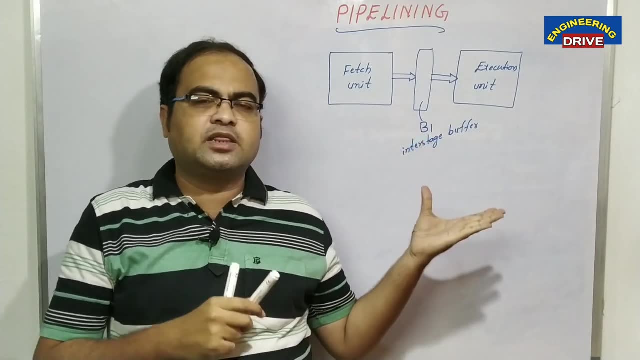 Ok, Ok, Ok, Ok. Before that, I am calling it as B1 buffer. So, with help of addition of inter stage buffer, what we need to do means we need to do small changes in the hardware of our computer to implement pipelining concept. 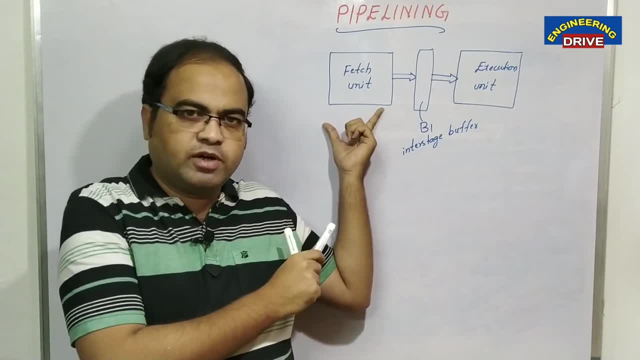 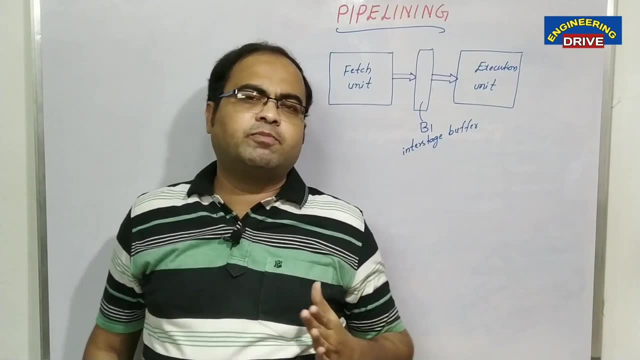 What we need to do. for fetching of instruction, there should be a separate hardware module. For execution of instruction, there should be a separate hardware module in between. then there should be a one buffer. You know what is a buffer? Buffer is a temporary storage place to store some data. ok. 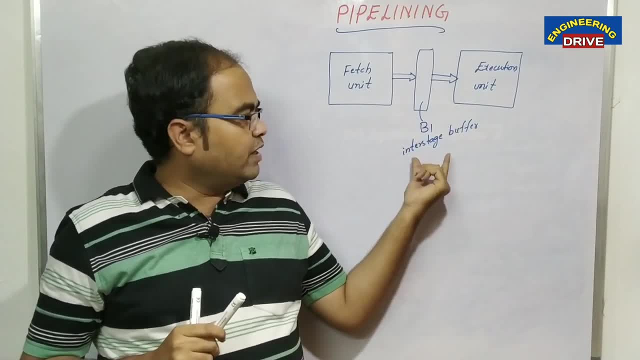 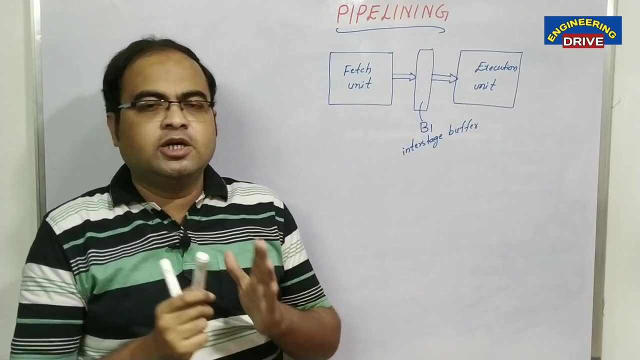 To store temporarily the data. we are using one buffer, B1.. Why we are calling it as inter stage buffer? because it presents between the two units, between fetch unit and execute unit. So what happened? how the pipelining concept will work. This is a hardware organization. 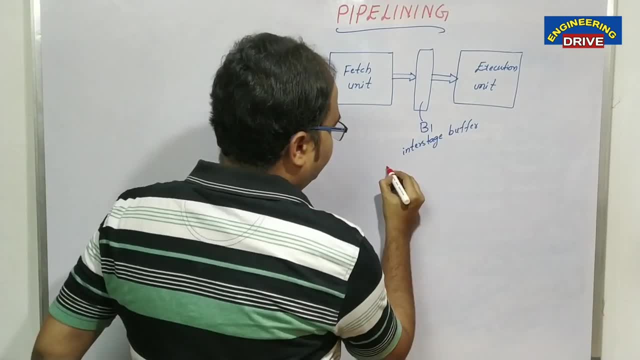 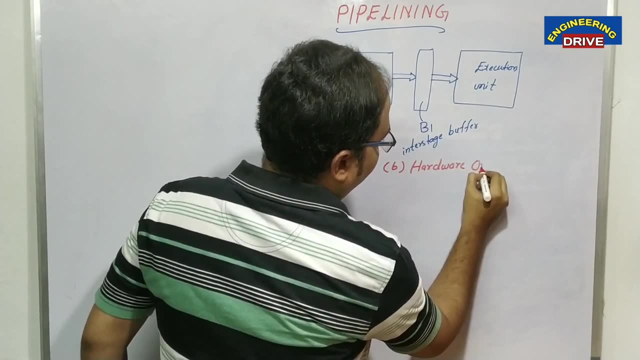 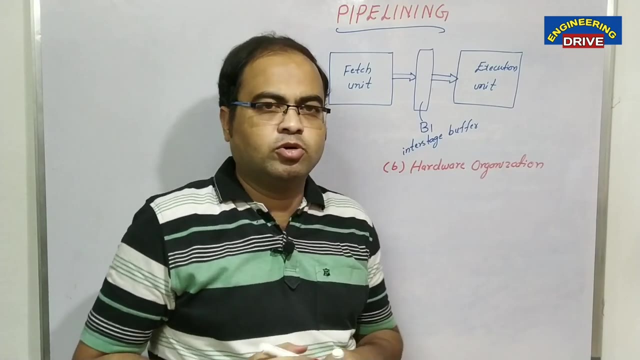 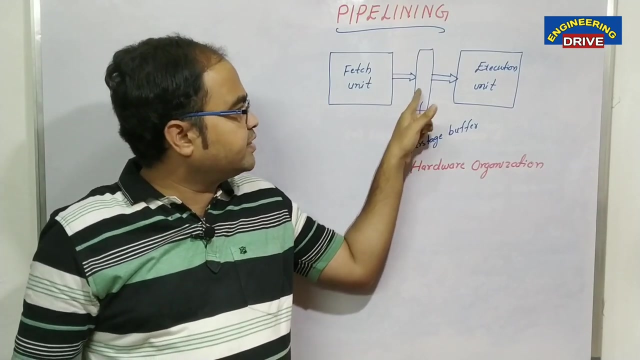 Ok, let me explain the hardware organization, then I will tell one example. This is a, this is diagram number B, hardware organization. Ok, so, my dear students, what happened? you know what is the job of fetch unit. Fetch unit will fetch the instruction as soon as the instruction has been fetched. that instruction. 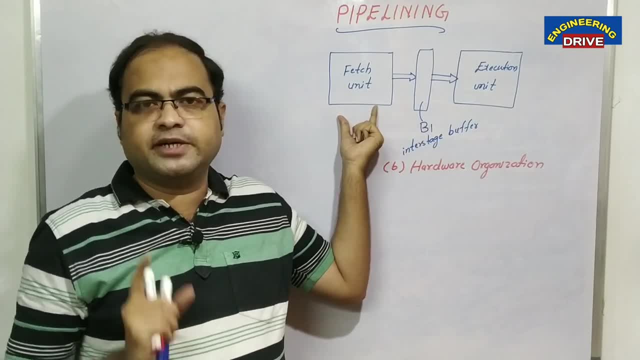 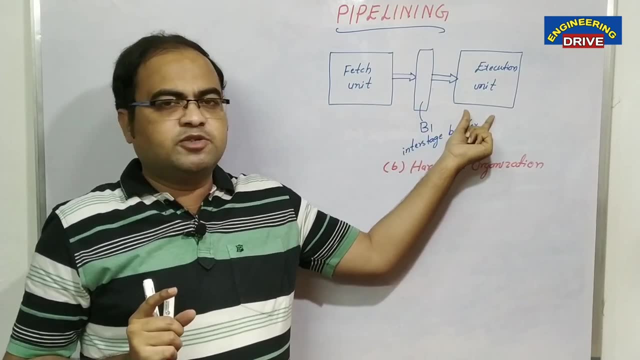 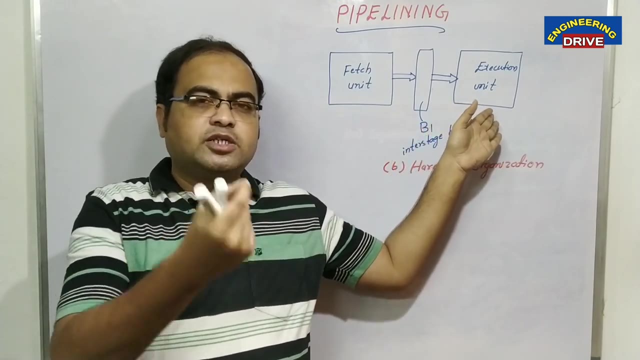 will be stored in this buffer B1, which means fetch unit is free. now, When the data is available in the buffer B1, whenever execution unit is free, it will take the data and it will start executing that instruction. Meanwhile, when execution unit is starting to execute the instruction simultaneously, 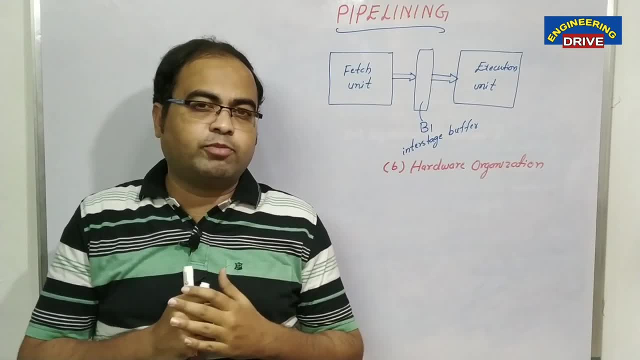 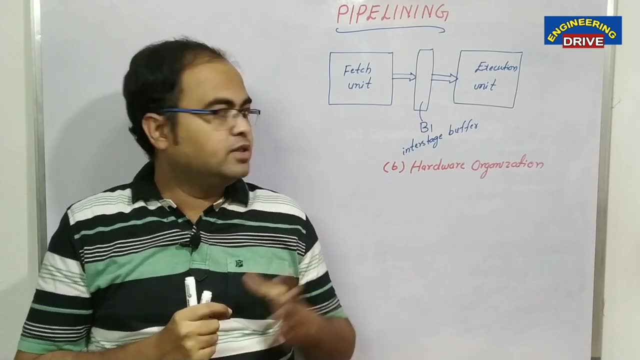 fetch unit will be stored in the buffer B1.. So what is the job of fetch unit? Fetch unit will fetch the next instruction. which means you can observe one point here: concurrent execution of steps is going on here concurrently, multiple instructions are being executed, yes or no. when fetch unit will fetch the instruction, it won't keep it itself. 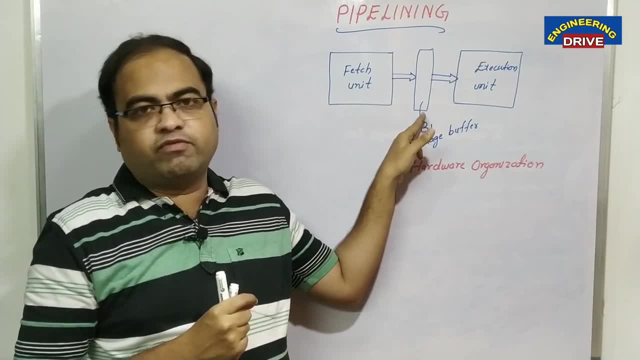 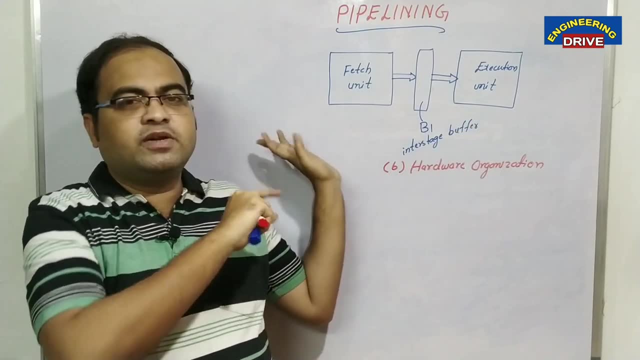 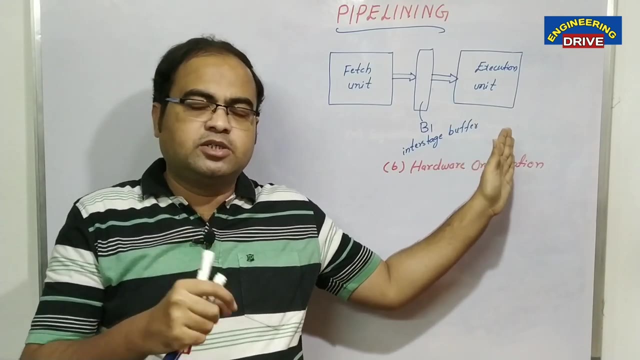 it will keep the. it will simply transfer the data to the buffer. What buffer will do? it will transfer the data to execution unit. when execution unit is executing the instruction, fetch unit will fetch the next instruction. which means, instead of fetch unit should become ideal Until the execution unit should complete execution of the instruction. fetch unit also. 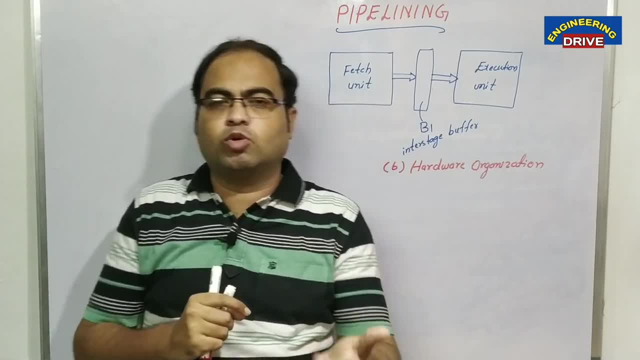 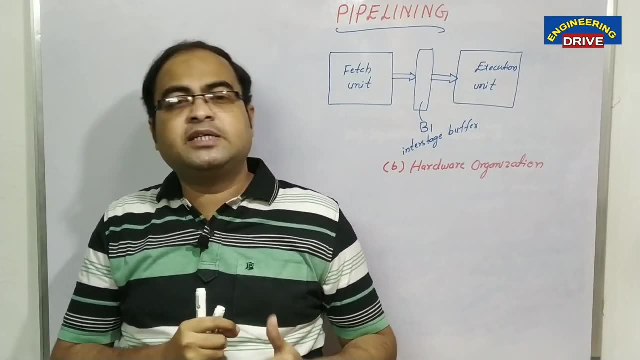 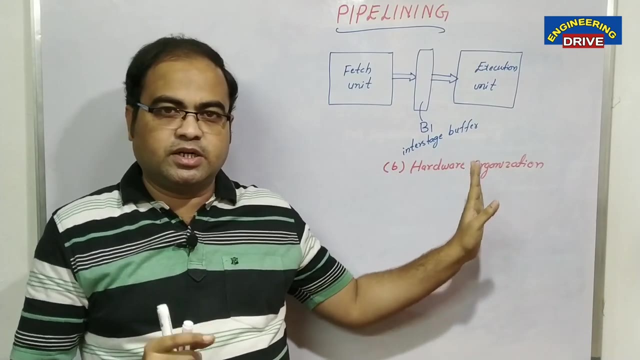 start working as soon as execution unit start its role of execution of instruction. So in this way, we can able to utilize the time of the processor. multiple instruction can be executed, which can improve the concurrency of execution. ok, This is hardware organization. now let me give one last example. now, with this, you can able: 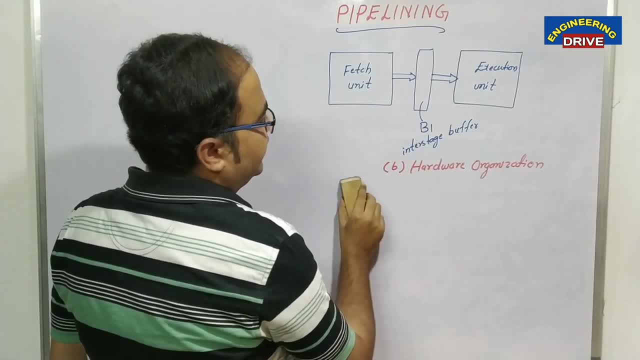 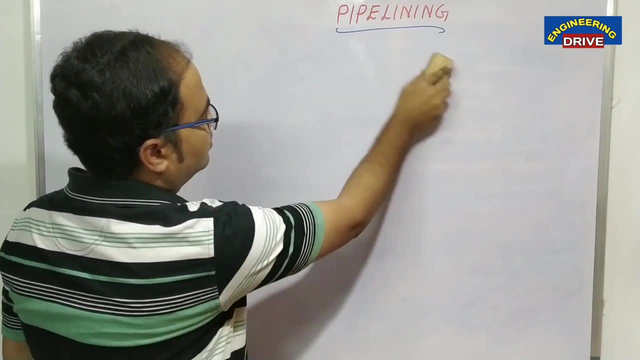 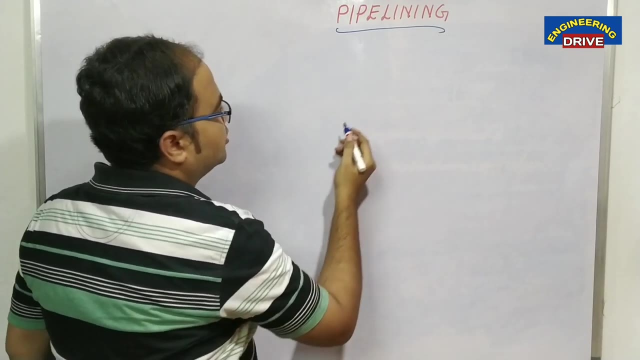 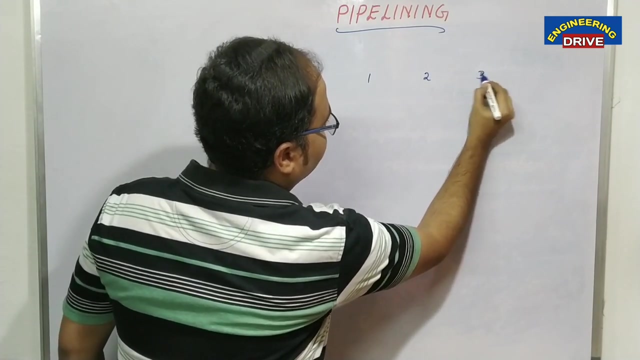 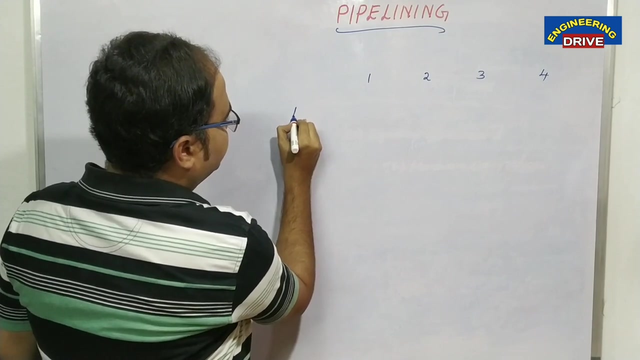 to understand how this Pipelining concept will work. now, this is hardware organization diagram. ok, let me erase this one. Now, my dear students, let us say: this is cycle one, cycle two, cycle three and cycle four. So what I am going to do means here, and this is the instruction one: 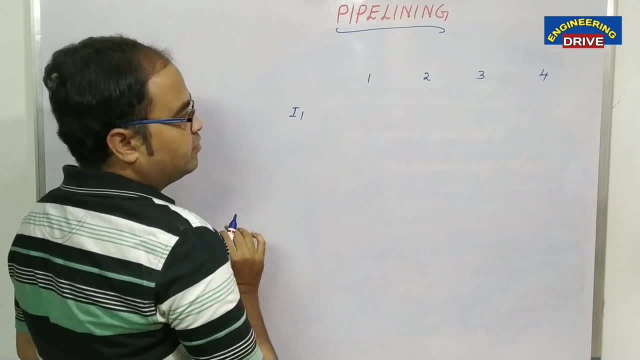 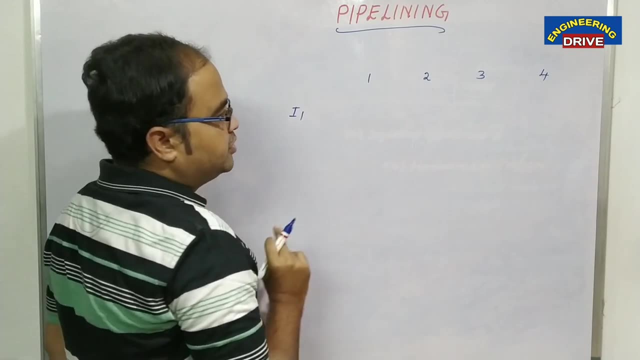 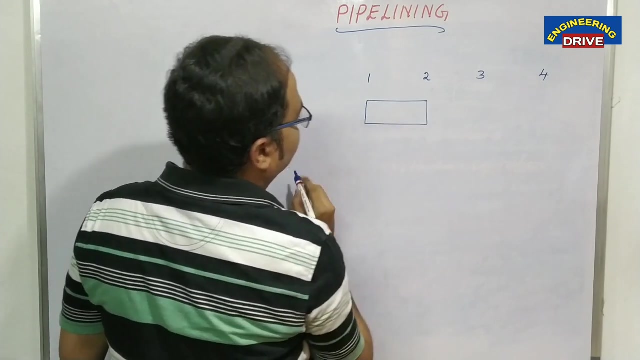 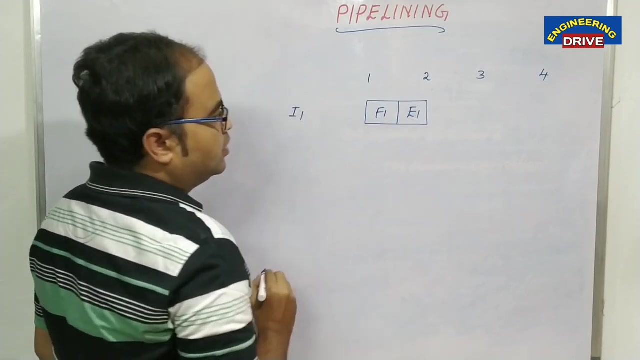 First of all, how I want to execute instruction one, how the instruction one will be executed. let us see. you know that in the execution of instruction we have taken two steps: fetch, fetching the instruction, execution of instruction. so what I am going to do- F1, E1. so instruction one will be fetched and instruction will be. instruction one will be. 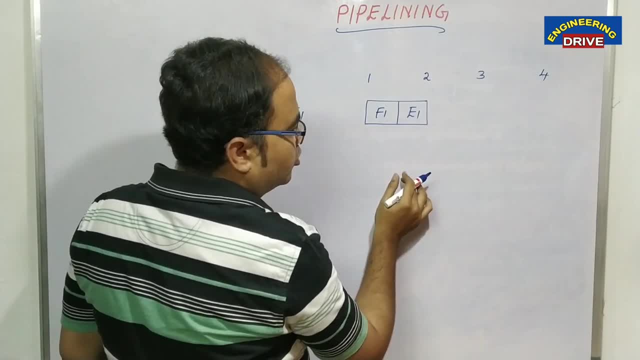 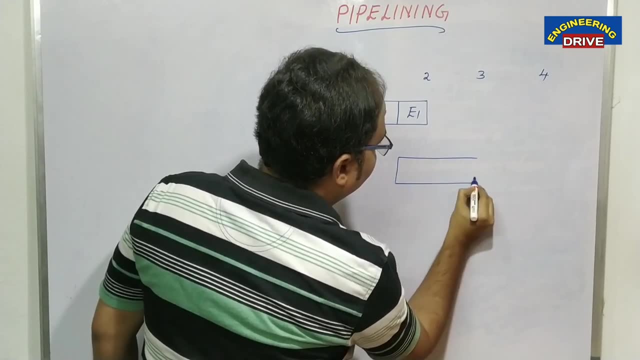 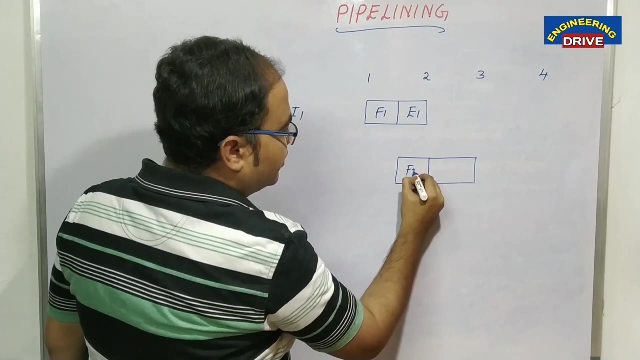 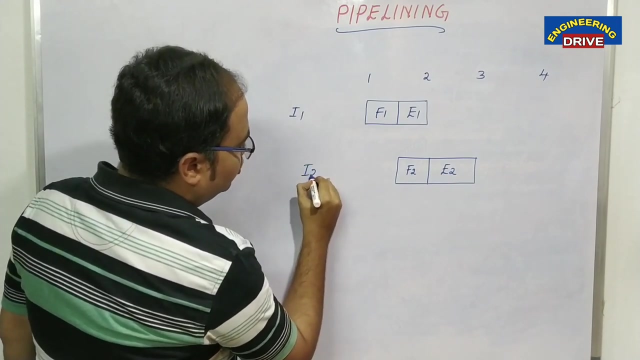 executed. during the execution of instruction one. what happened, you know here, During the execution of instruction one, Instruction two will be fetched and instruction two will be executed. this is in case of instruction two, F2., F3., F5., F6.. 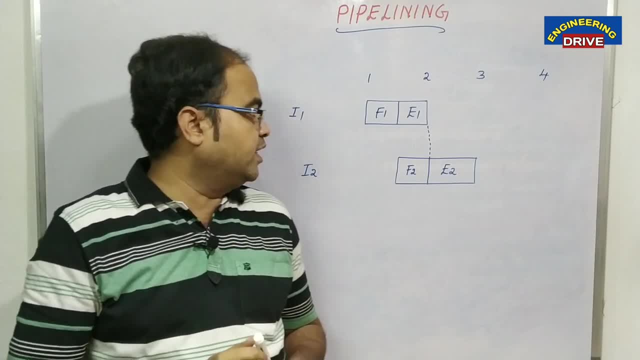 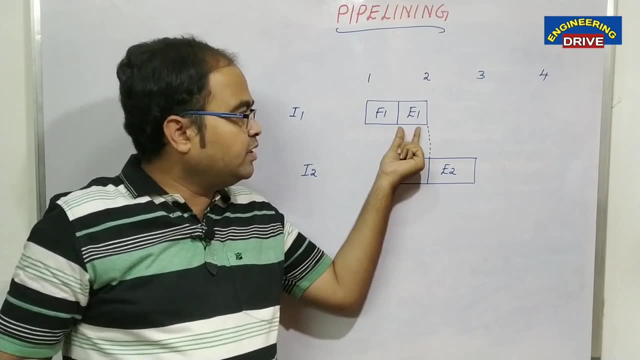 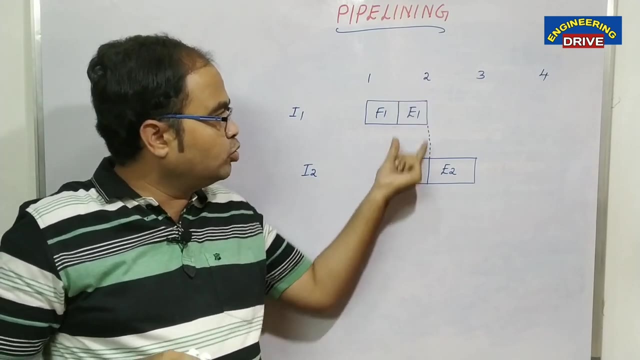 F7.. F6.. F7.. F8.. F9.. my dear students, hopefully you will understand now. see here: instruction 1 will be fetched and executed normally, but during when the instruction 1 will be. during the execution of instruction 1, instruction 2 will be fetched during this time interval only at the time interval 2 at the cycle. 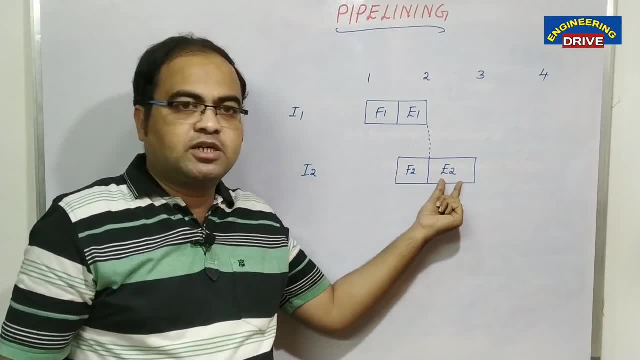 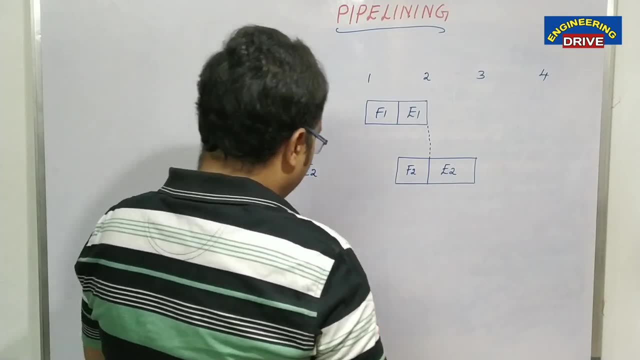 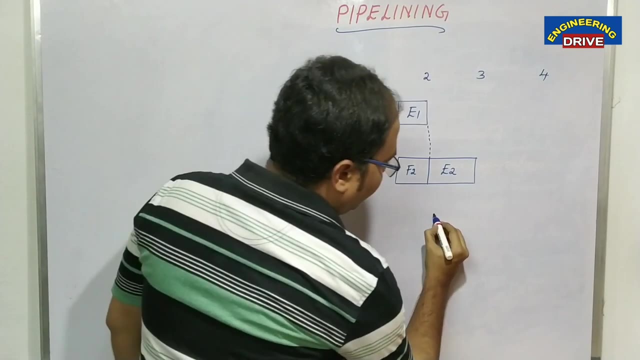 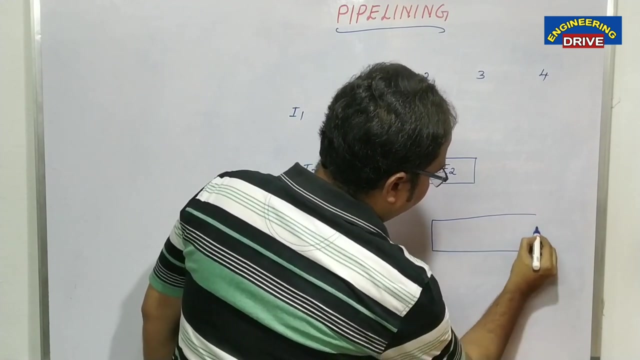 2 itself. instruction 2 will be fetched and then instruction 2 will be executed in cycle 3. now what happened, you know. next step, let us say one more instruction is there, i3. now can you to guess what happened in i3? i3 fetching will start from here. fetching of third instruction. 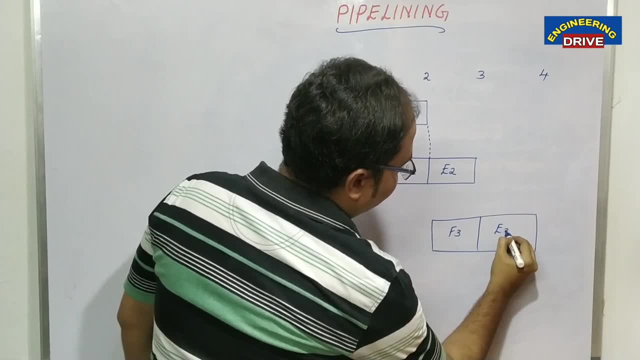 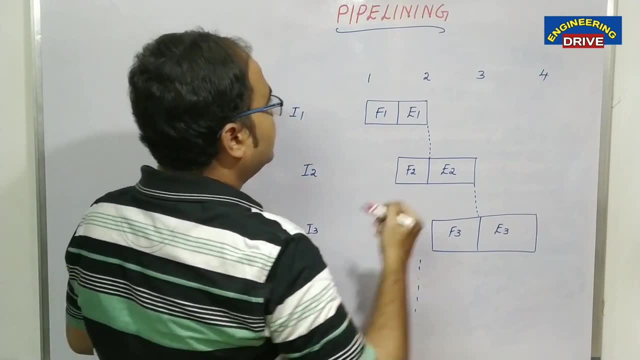 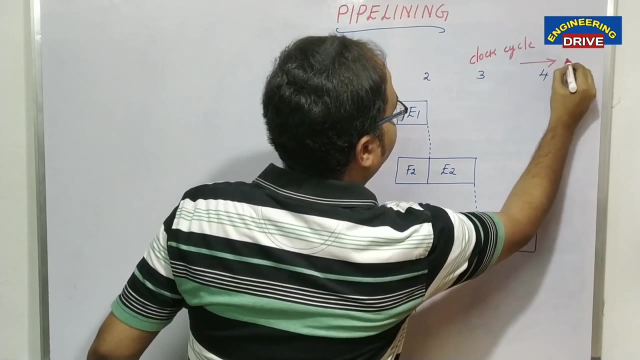 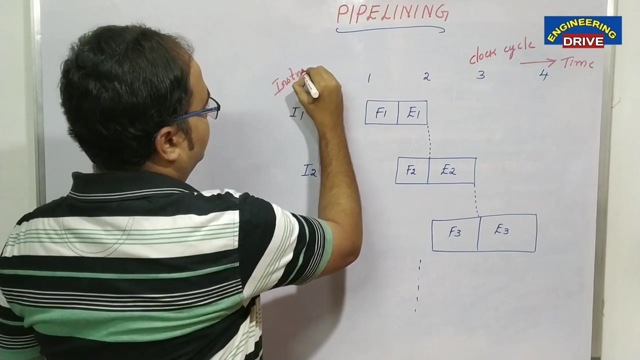 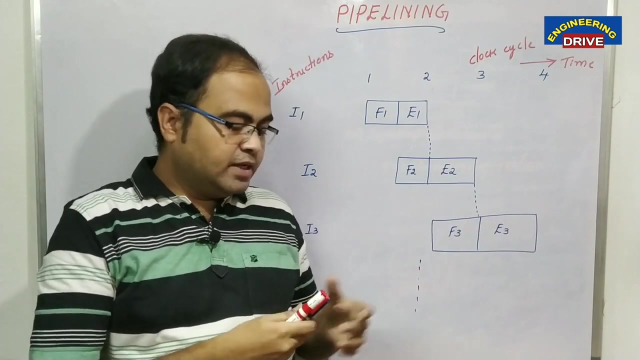 and execution of third instruction, and so on. okay, this is nothing but our clock cycle, this is our time and these are nothing but our instructions. so, my dear students, now you see, this is a this is diagram, will speak about, about for you, and this diagram is nothing. 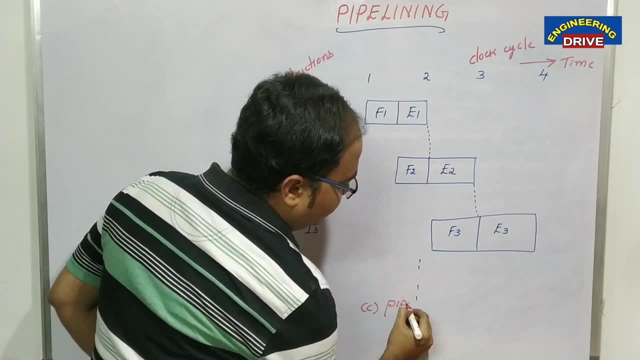 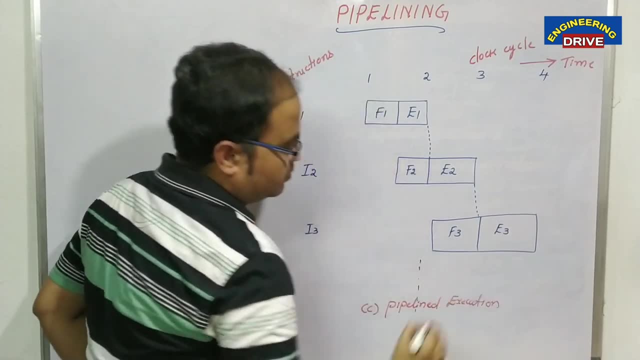 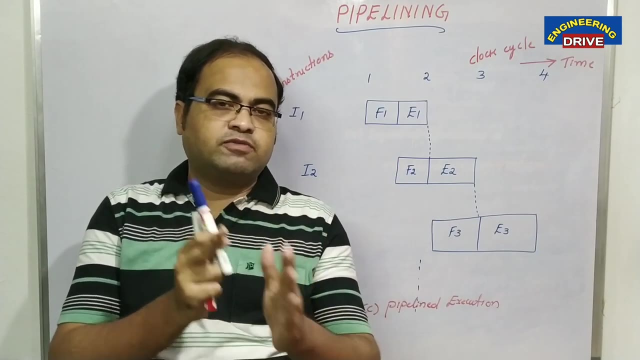 but our instruction. so, my dear students, now you see, this is a diagram number C. this is our pipelined execution. First diagram which I have told you is sequential execution: F1, E1, F2, E2, F3, E3, yes or no. So, after instruction 1 is fetched, 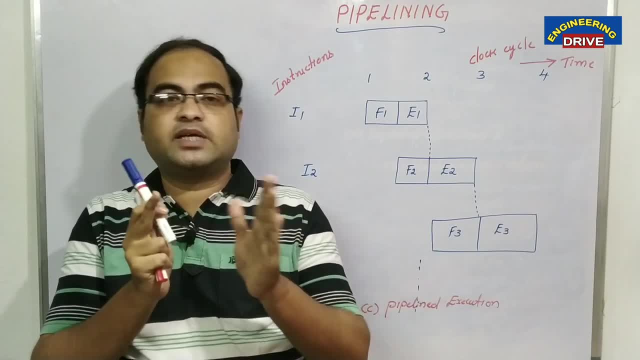 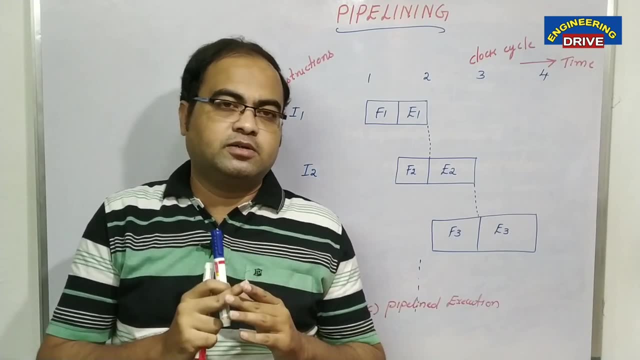 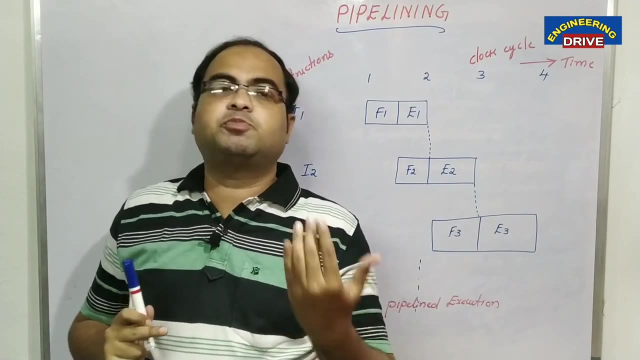 after instruction 1 is executed, then only the fetching of second instruction will start. Once the second instruction is being executed, then the fetching of third instruction will start. But in pipelined execution it is not like that The concept of pipelining is: we want to increase the speed of our computer. 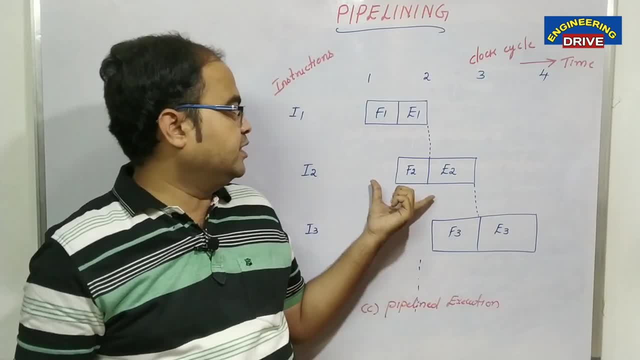 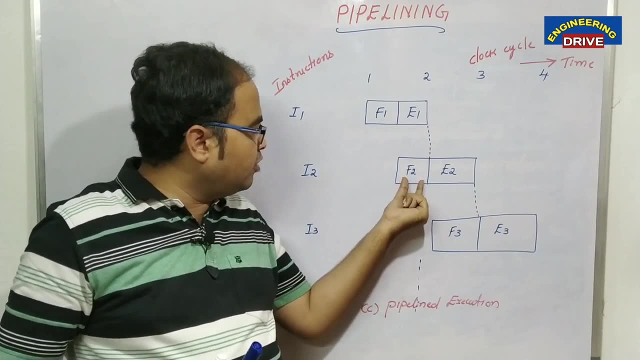 we want to achieve concurrency. How we can achieve concurrency Like this? only When instruction 1 is being fetched and executed during the execution of instruction 1, fetching of instruction 2 will start. Now you can see concurrency is there here, Yes or no? Similarly, 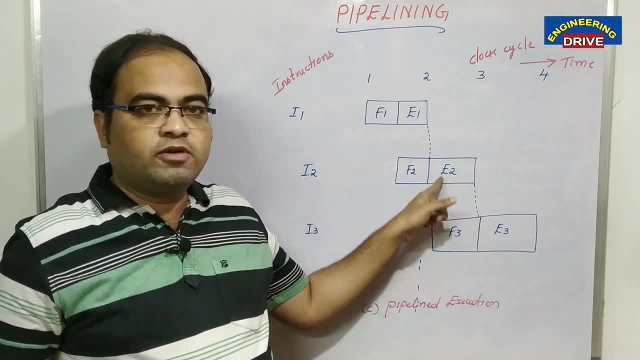 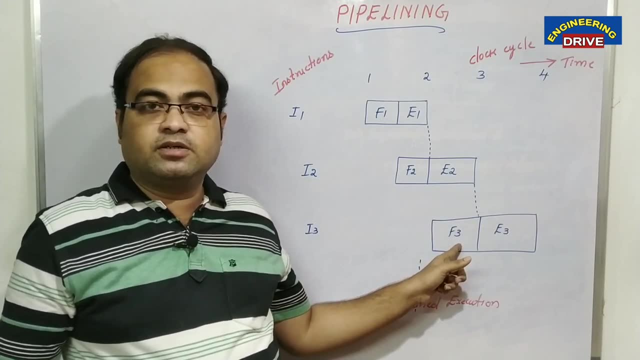 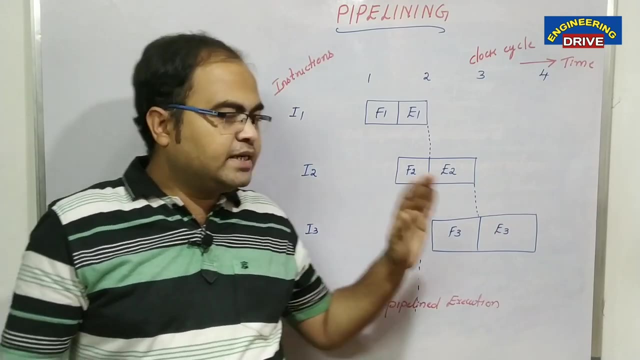 when the instruction 2 is being executed, during the execution of instructor instruction 2, fetching of 3rd instruction will starts, will be started here, So which means when the instruction 2 is being executed, instruction 3 is being fetched. Now let us say one more instruction. 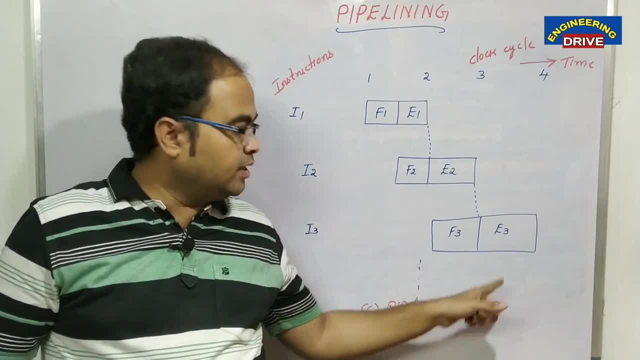 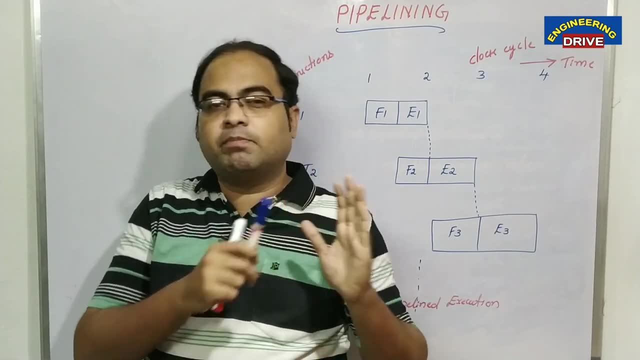 is there instruction 4. what happened, from where it will start is fetching. when instruction 3 is being executed, fetching of 4th instruction will start like this. So in this way, what happened? And compared to the sequential execution, pipelined execution will have a lot of benefits. 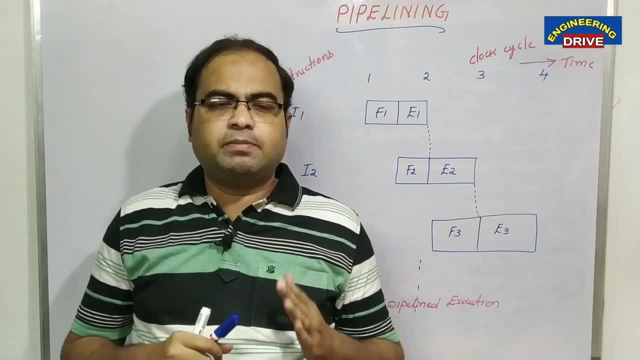 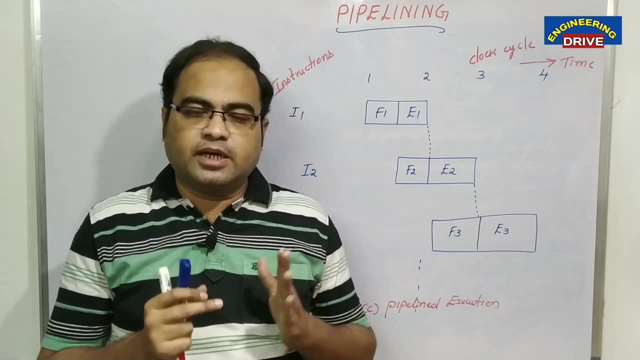 What are those lot of? one of the big advantage of pipeline concept. pipelining concept is the performance of our computer will drastically improves. okay, Why it will improve a lot? The main reason is the concurrent execution of the instructions. that is the answer. 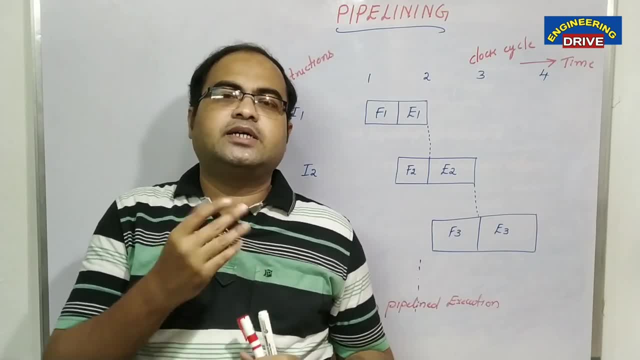 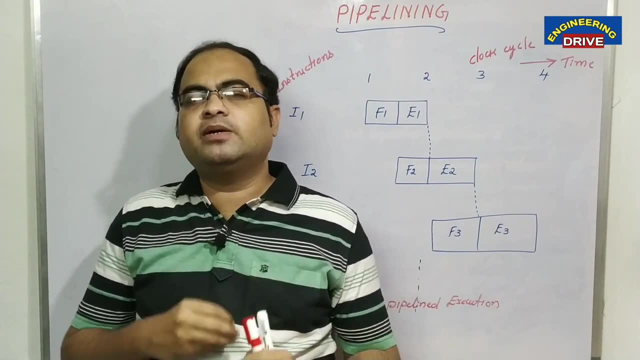 So pipelining is a concept which is used to establish concurrent execution of instructions in our computer. okay, And the major drawback of pipelining is you need to implement more hardware in our system, So it will be very expensive approach, but the main big advantage is the performance.